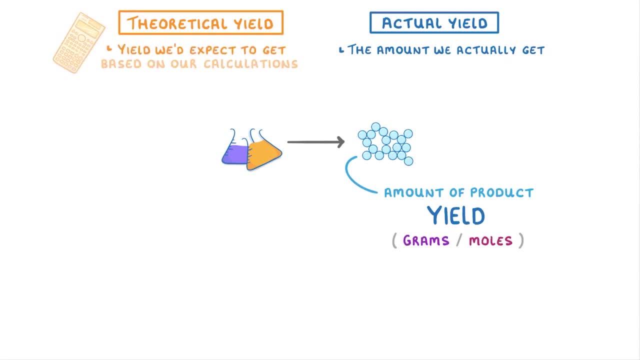 yield to describe the yield we'd expect to get, based on our calculations. For example, if we reacted 2 grams of hydrogen with 16 grams of oxygen, then we should get 18 grams of water. So that's our theoretical yield, because 2 plus 16 equals 18.. 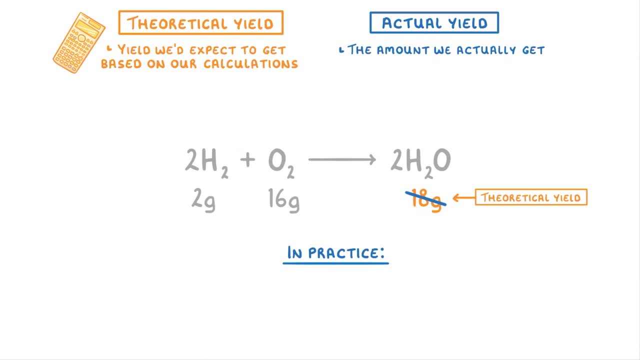 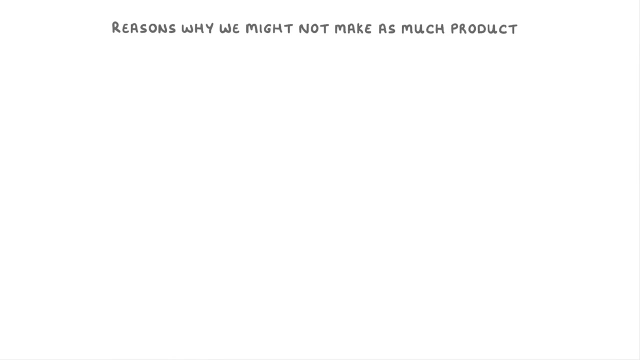 In practice, though, it might not make quite that much. For example, we could end up with only 50 grams of water- 15g or so- and we'd call that our actual yield. Now there's a whole range of reasons why we might not make as much product as we expect. 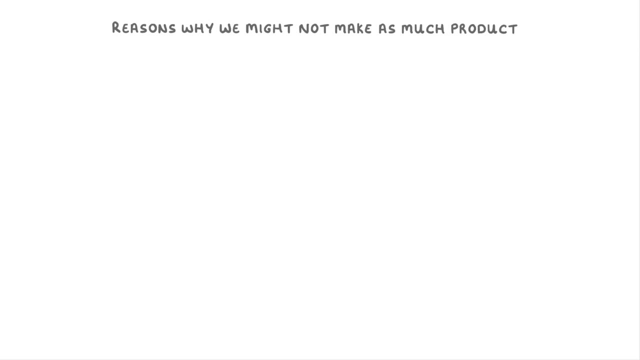 but there are three particularly common ones that you need to know. The first is that the reactants might not all react, so at the end some of the mixture will still be reactants. This could happen if the reaction is particularly slow, so it just hasn't had enough time. 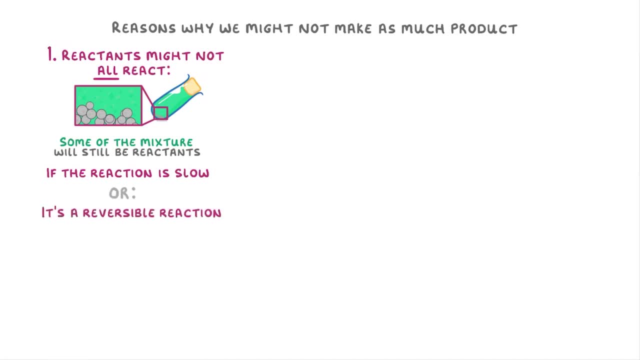 to fully react or because it's a reversible reaction and it's reached equilibrium. For example, if we reacted nitrogen and hydrogen to make ammonia, it wouldn't ever go to completion because it's a reversible reaction, so some of the ammonia would keep breaking. 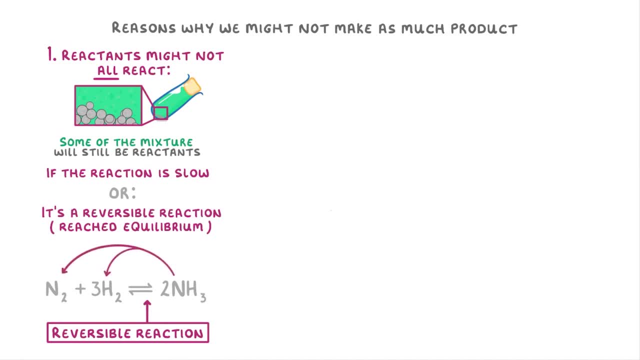 back down into nitrogen and hydrogen. The second reason is that the reaction is slow. The second reason is that the reaction is slow. The third reason is that there could be side reactions, which is where the reactants react to produce a different product than the one that we were expecting. 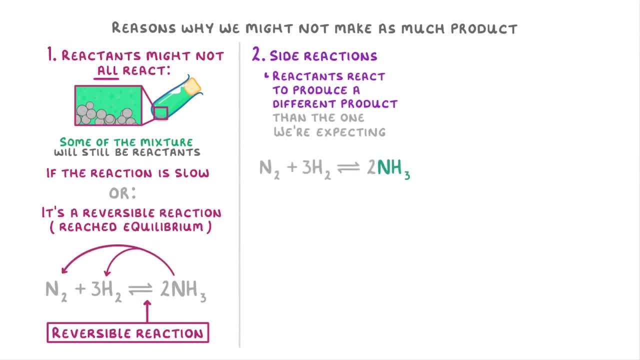 For example, if we were looking at the same reaction as a minute ago, some of the nitrogen might react with oxygen from the air to make nitrogen dioxide instead of going to make ammonia, like we wanted it to, and so we'd end up with less ammonia than we expected. 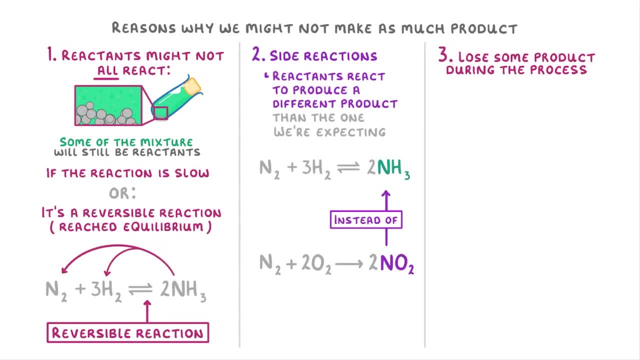 The fourth reason is more simple. We could just lose some of the product during the process. For example, gaseous products can float off and escape. Or if we were filtering something, we might not capture all of the liquid or solid. To understand what we mean, imagine that we were using a filter paper and funnel to filter. 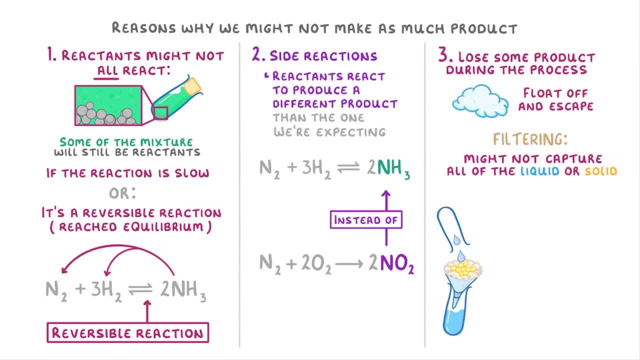 out a solution and separate the liquid and solid. If our aim was to capture all of the liquid and solid, we might not have captured all of the liquid and solid. If our aim was to capture all of the liquid and solid, we might not have captured all of the liquid and solid.